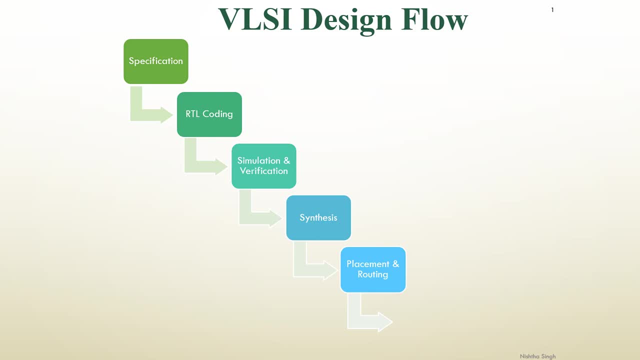 place the logic elements or the gates, or whatever the flip-flops are there in your circuit components, where to place them, how to utilize the space of the whole chip so that the space utilized is also less, and this is followed by routing. so in this step. so whatever the components you have, 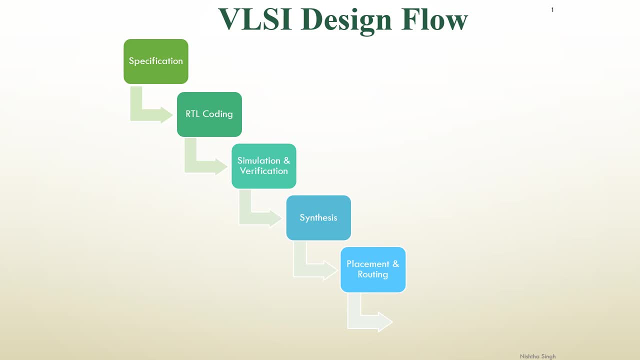 placed on your chip. you need to provide a path also how the data is going to flow from where to where. so that path is decided by routing step. so the last step is manufacturing the chip, whatever the design you have proposed and whatever the design you have designed. so now the next question. 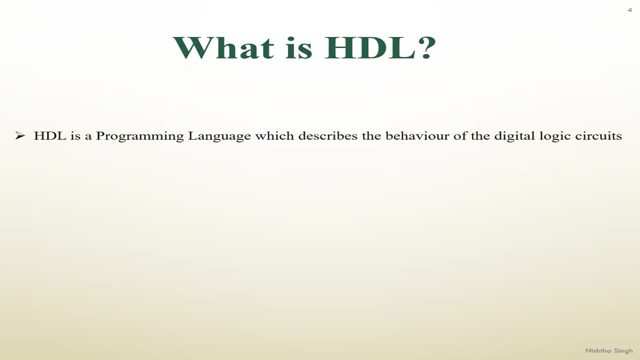 that comes in our mind would be: what is hdl and why do we exactly need hdl? so hdl is not directly a process, but it is a simple programming language. so we can say that hdl is nothing but a simple programming language which describes the behavior of any digital logic circuit. so hdl is 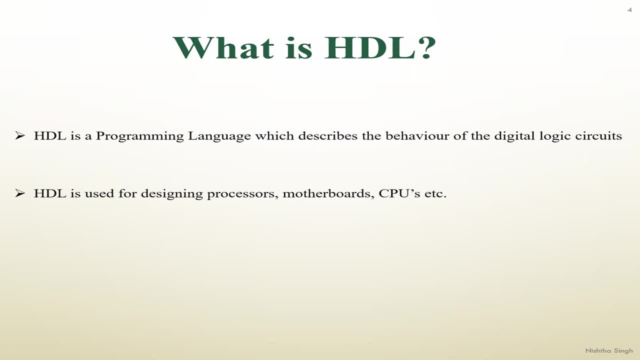 used for designing all the processes and motherboards that there that are dead in your laptops or in your computer systems. they all the chips that are designed. they all are done using the hdl only. so there are basically two types of hdl. one is verilog and the other one is 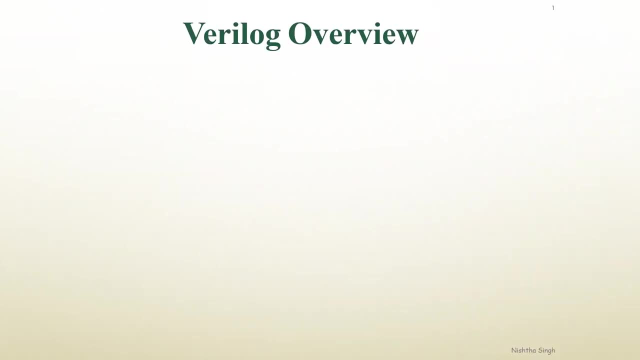 vhdl. so in this lecture we are going to be about Verilog. so Verilog, as I told you guys, is a hardware description language and Verilog is an IEEE standard. also, this is IEEE 1364. Verilog is a concurrent language, unlike C language, which is a sequential. 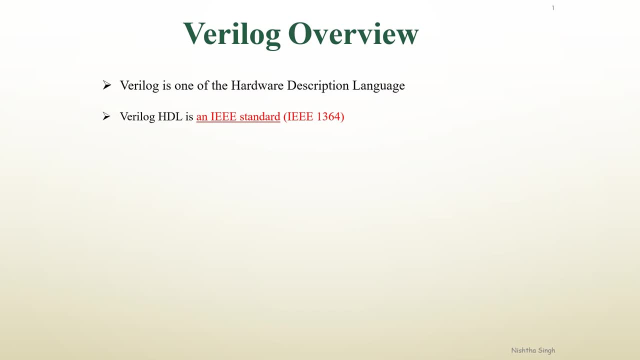 language in this. all the statements that are written in this Verilog coding all will run at the same time. they are not going to wait for the first statement to execute and then the second statement is going to wait. so this language is also a case-sensitive language. so, as I told you before that it 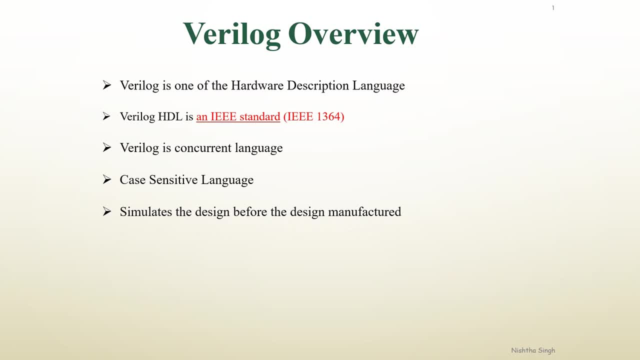 simulates the design before the design is manufactured. so the simulation guarantees that the design behaves as it should be, the functionality of the design is correct and it also provides three basic modeling styles, that is, behavioral, structural and data flow. so all these three styles I am going to 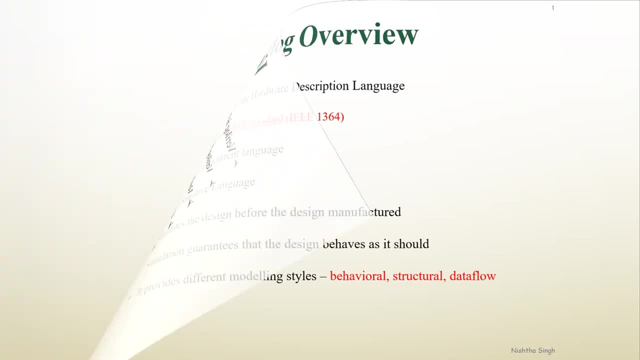 cover in my future lectures. so stay tuned for that. so now I'm going to tell you the basic program structure that we are going to cover in this lecture. so let's start with the basic program structure that is there in the Verilog. so the first line that you have to write in any while writing any Verilog program is: 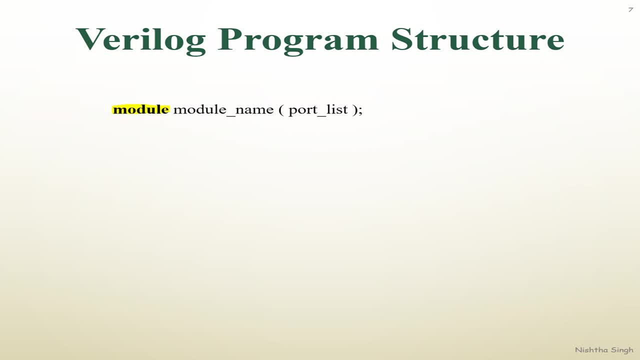 is this line, that is module and this is a keyword that specifies that you are going to write any module now and then you have to write the name for the module and then also you have to enlist whatever the ports are going to be there in your module or in your design, like whatever the inputs have or the outputs. 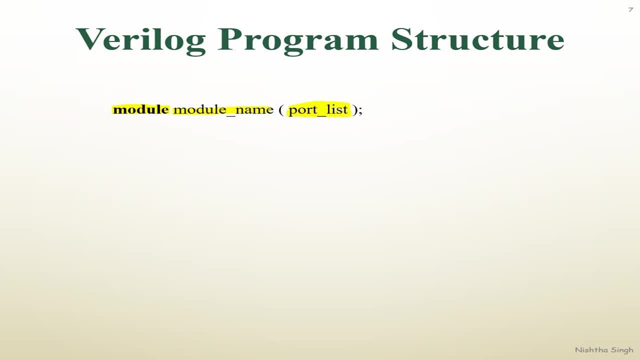 and then you have to write the names over here- this is known as the port list- and then the next step is port declaration. you have to declare whether that particular port is input or the output port, and the next step is declaring any variable that you are using. and the last step would be the. 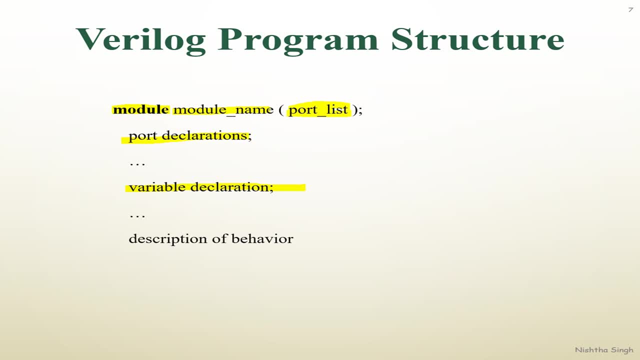 description of behavior, like what the functionality of the chip is going to be or your design is going to be. you have to write all the behavior of this design over here and then end it with end module. so, for example, let us take an example- so here I am taking an example- of a NOT gate. so this: 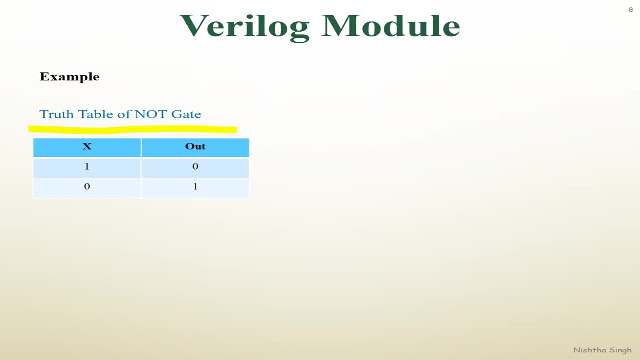 is the truth table of the NOT gate. so when the input is 1, you get an output 0 that is inverting. so the function of the NOT gate is to invert the input. so whatever input you are going to give, you are going to get an inverted output. 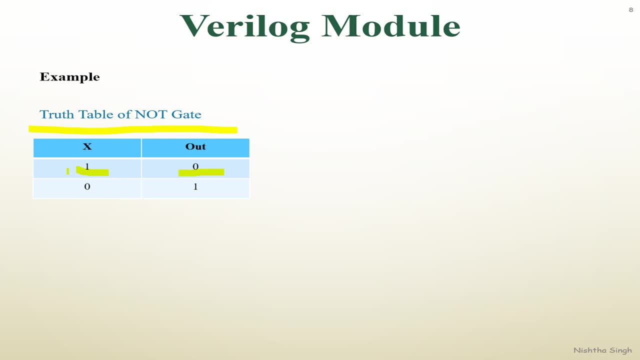 right. so when you are giving 1, so the output will be 0, and when you are giving 0, so the output will be 1. so this is the basic gate, like this, and now we are going to start the coding. so first you have to write the. 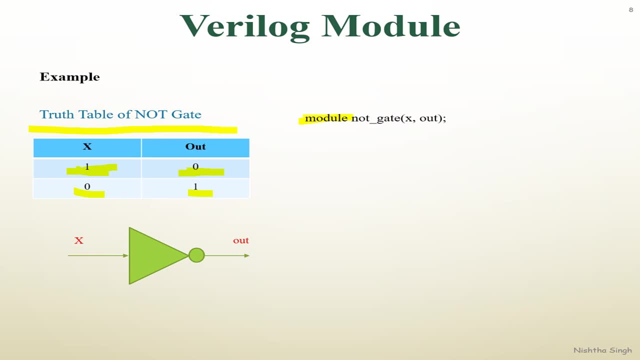 module keyword, as I told you in before slide, and then you need to give the name for the module- so I have given here, NOT underscore gate- and then, as I told you, you have to need to enlist the ports, whatever the ports are going to be in the module. so now you can see from here that it has only one input, a, NOT gate. 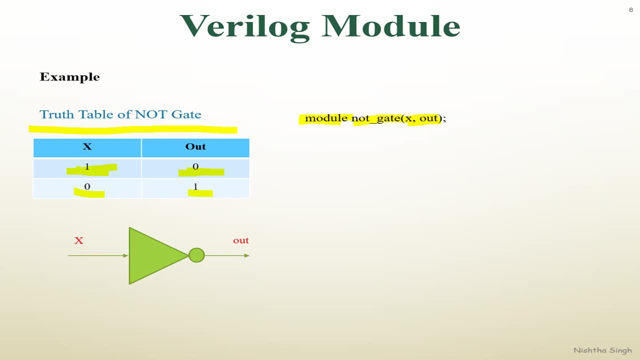 has only one input and has one output. so that's why I have written here: one input and one output. you can declare the variables, okay, and then this is known as the module declaration. then next you have to declare the input and the output ports, like you have to declare which variable that port you. 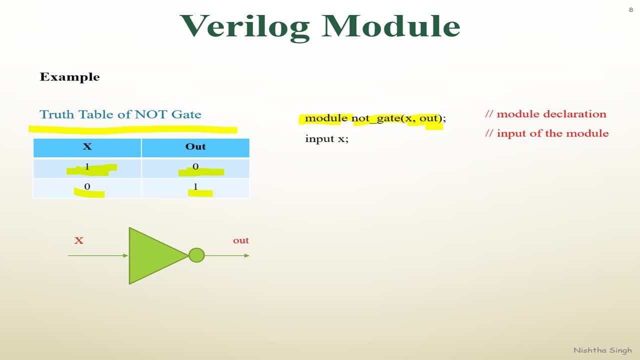 have written here whether it is input or output. so here I am giving this X as an input and then output is OUT. okay, so now, as I told you, you have to describe the behavior of the module. so here, this is what I am doing here. so now, here what I am doing: I am assigning. 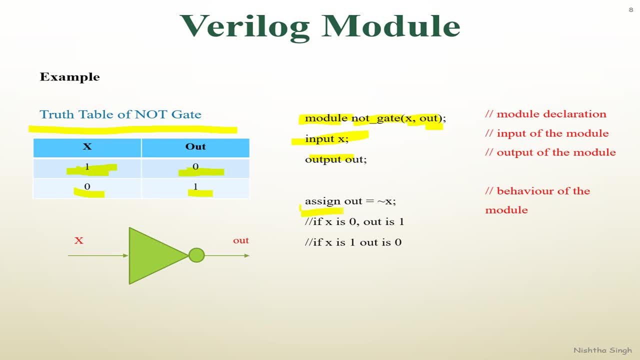 the out. so whatever my output is going to be, it has to be inverted of the input. so for inversion you need this symbol. this is a symbol for inverted. so when this particular statement is written in your code, this means that you are going to invert the input, you are performing a NOT gate function, and then you can. 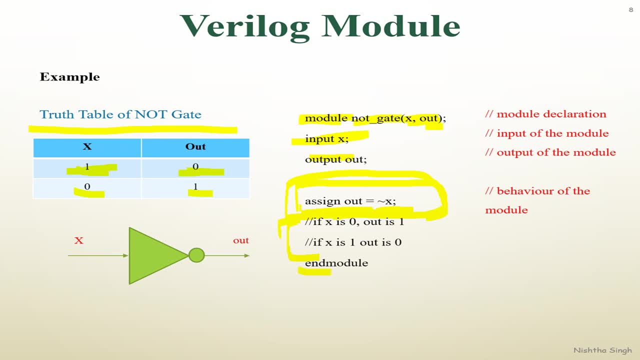 also give the comments over here. this is the comments, and then in the end again you have to mention AND module. this is the basic method of how you have to do the coding in the Verilog. so now I'm going to tell you how to download the. 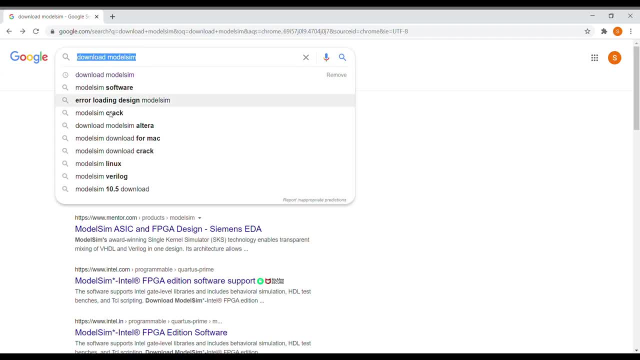 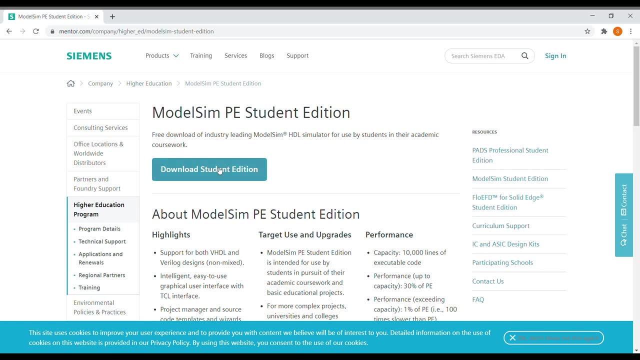 冷 ajudar mod modernizedmitual model sim library. so you just need to go to google and then write download mod vive model sim library and then the first website you have to click on this mental graphics website and after downloading you just need to install the installation. 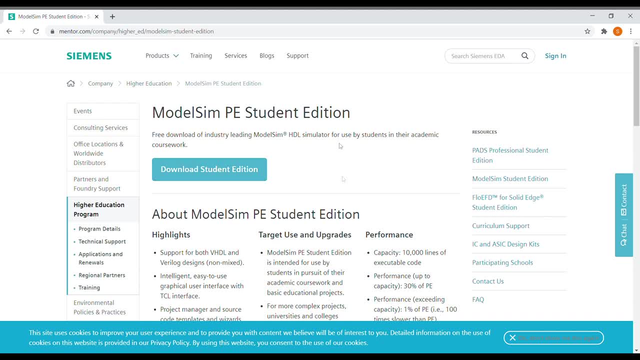 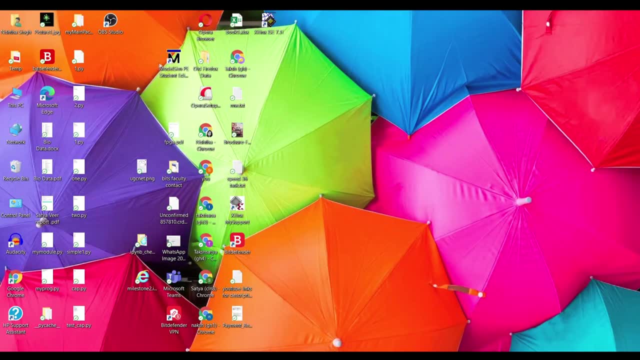 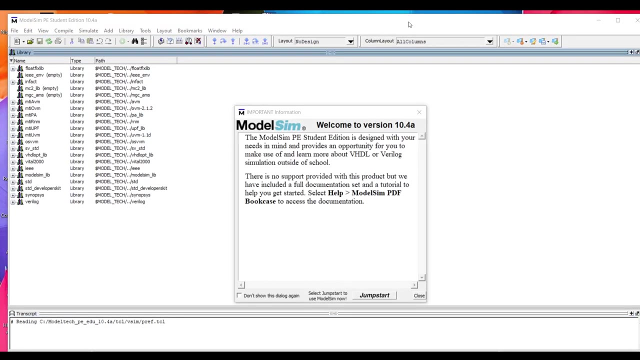 process is also is also very simple, so it is already installed in my laptop, so i'm not going to demonstrate that. so now, once you have downloaded and installed the model sim, now you can just go to the desktop and you will find an icon like this, over there written m, and then just click on that icon and the model sim will. 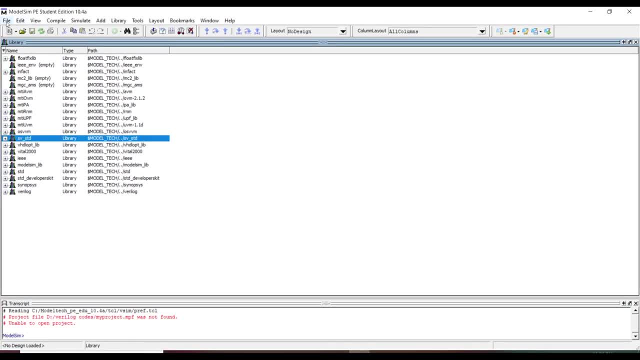 launch. so this is how the model sim environment looks like. so now i'm going to tell you how to start your new project in this model sim, to do the coding so you need to go to the file menu and then select new and then select project option from there and then a pop-up window will open. 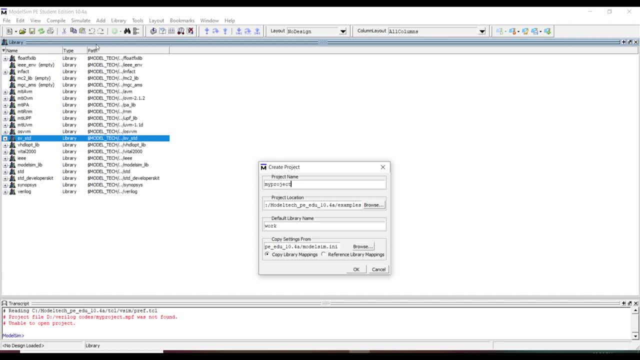 and there you have to write the project name- any project name you can give. i am giving here my project- and then you also have to select the folder, destination folder where your project you are going to save it. so i am just selecting that. so now, once that is done, you need to click. 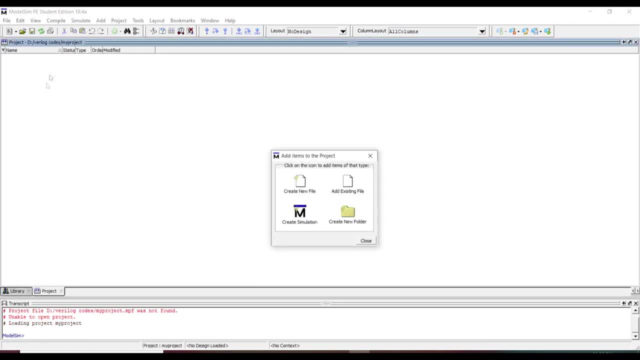 樂. okay, and then you can see here that your new project is open. a new window is open, you can see the project name and the path. also you can see where you have saved the project, and then you can also see a new pop-up window also there. so you are being asked to create a new file. 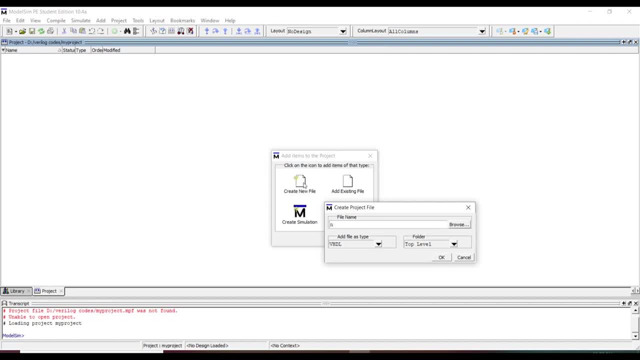 add an existing file or create a simulation. you need to create a new file from here for writing the code. so i'm just going to click on that and then i'm going to give a file name. so i'm giving- not underscore- gate, and then you also have to select the file type. so i'm here selecting very 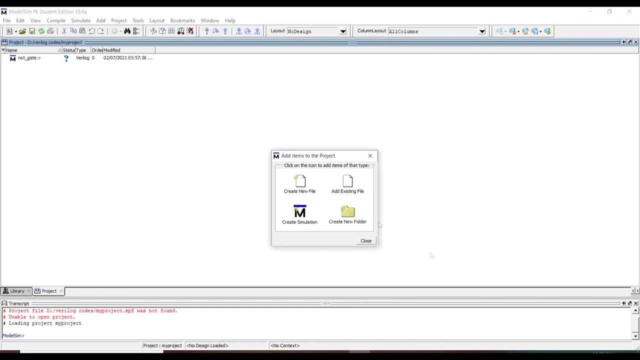 log, because we are going to write the code in very log. so now you can see that the file name is also there and the file extension is also dot v. dot v means that it is a very log file. now just double click on that file and the text editor will open. now you can. 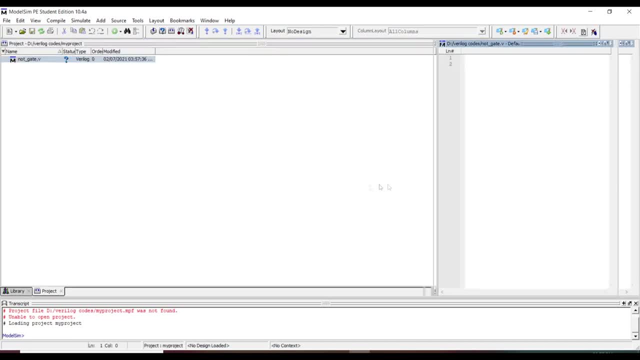 start writing your code. so i'm going to start. so I'm just going to write the code, whatever I explained in the presentation module, not underscore gate, then giving their port list and then declaring the inputs and the outputs and then assigning the behavior of the module, what the module is going to perform, and then just doing the end module. 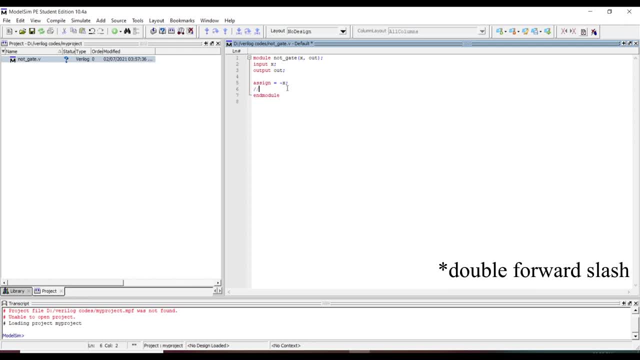 so if you want, you can also add the comments using the double backslash. then it will be easier to for you also to know, or for any other person using your code in future. then the person will know that what that statement or the module is performing. so you can add the comments like this: 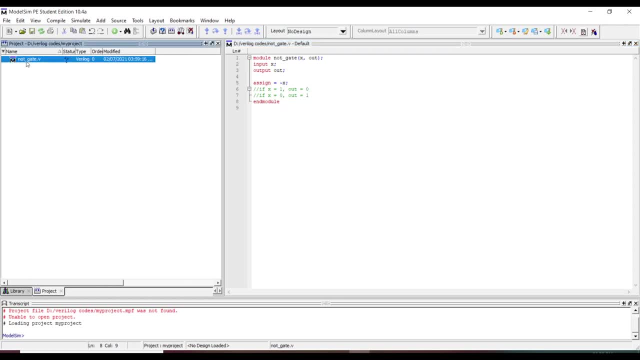 so now to compile the code you just need to click on right, click on the file name, and then you'll get a compile option. then compile the selected file and then now you can see that here that I am getting one error. I know what kind of error is that, so I just have deliberately have done that. 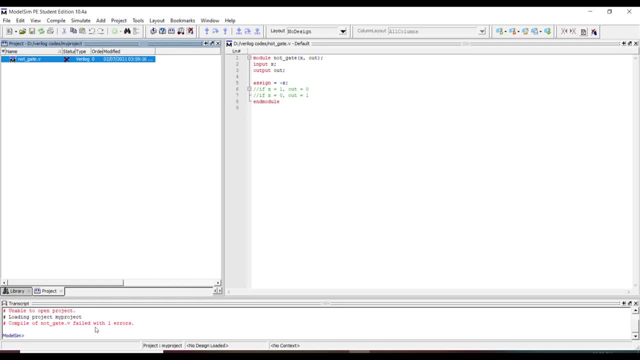 to show you how to compile the code. so now I'm going to compile the code and then I'm going to show you guys how the errors come. so here you can see that it is saying syntax error. so the error is that while writing the statement assign, I have not used the output variable. where I'm going to 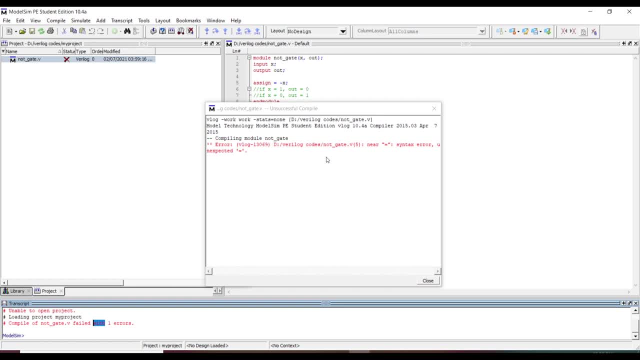 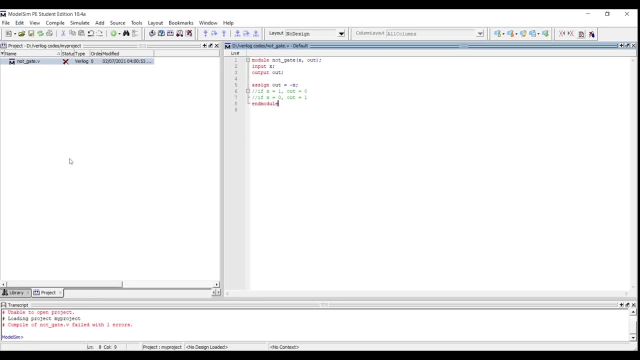 assign the input variable to. I have not used that, so I have to write that. so I'm just going to write that. so now my code is proper. I know it will get compiled without any errors also. so again doing the same process, compiling the, and now you can see that it has been compiled. and now you can see that. 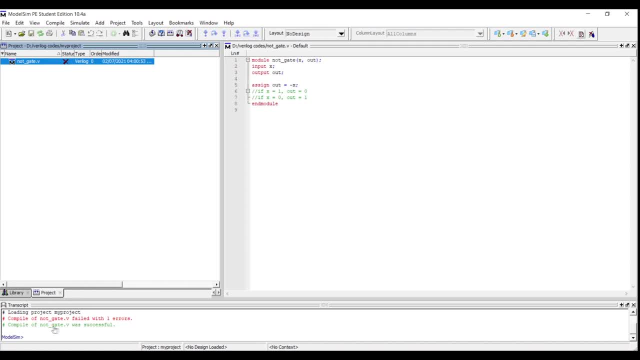 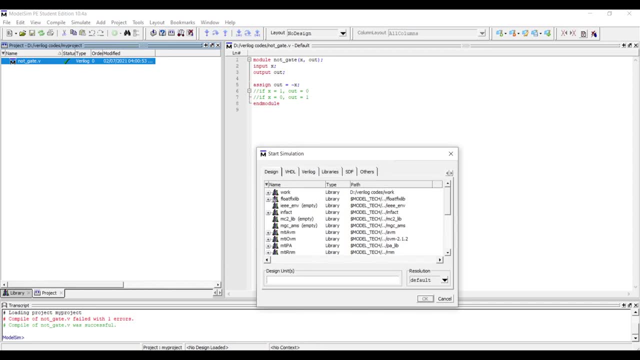 it has compiled and it is successful. now it is the time for simil taker built with the code. you would probably challenge the code, so to do that you need to start the simulation from this tenderly tab and then just click on the work folder over here and then click on the module. 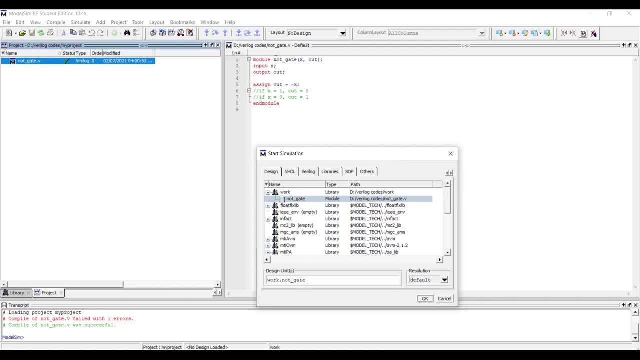 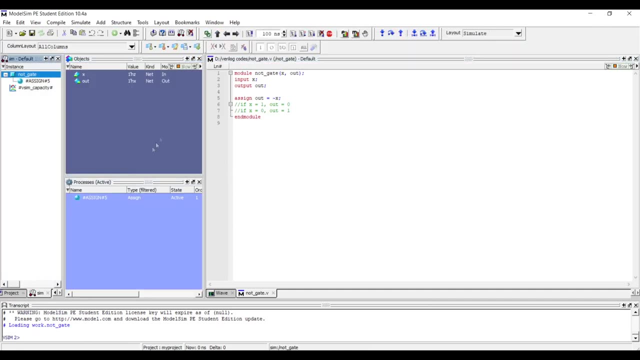 name. here you need to select the module name, the name that you have given. here in the module. they select exactly the same name, so it is not a routes for get. so now, if you can see that the object is open, it is showing me what are my input and what are my output. so now I 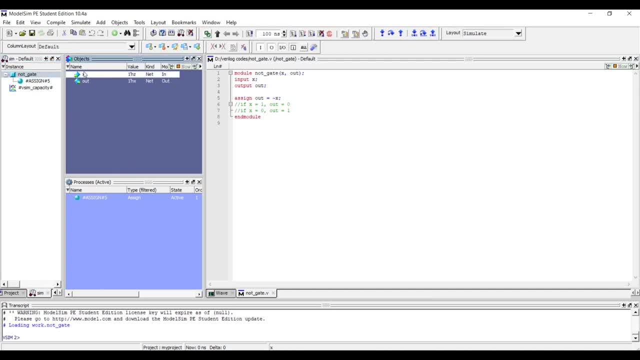 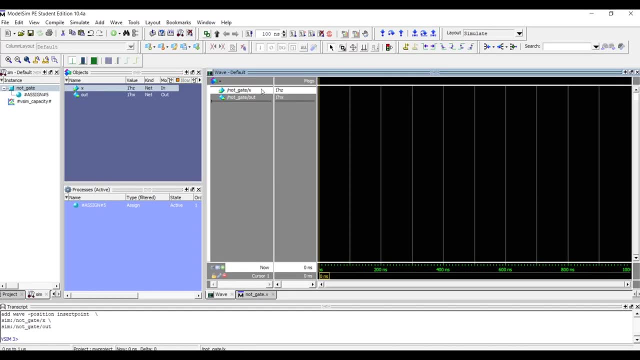 have to add those, both input and output, to my waveform to see the waveform, to see the functionality of the code. so now I'm going to assign the value to the input. I'm going to force a value to input. I'm just going to write 0, so I'm 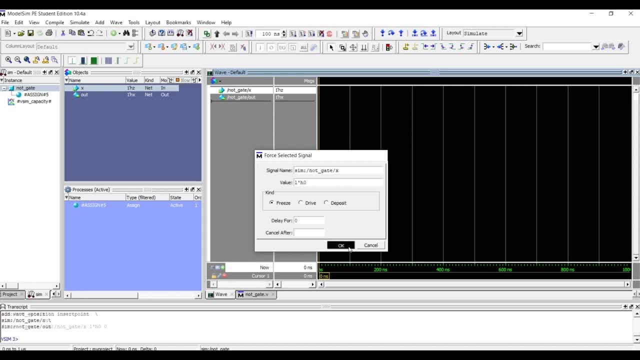 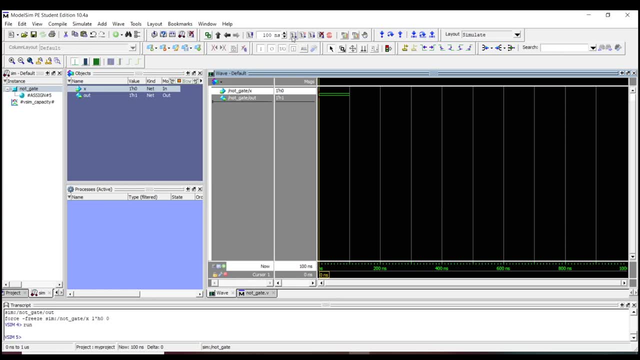 going to start with 0. so you can see, now I'm going to run the code for 100 nanoseconds. I'm there and let this 100 nanoseconds. now you can see. let me just zoom it for you guys. so now you can see that the input was 0 and the output that. 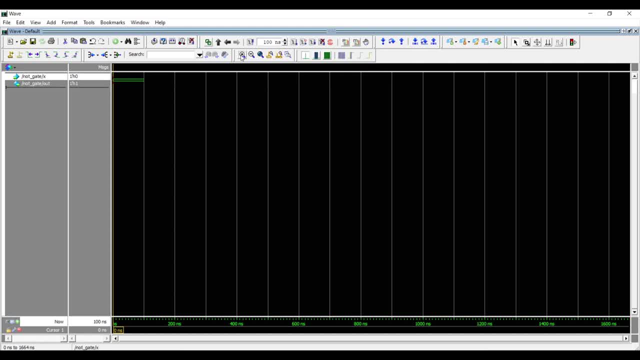 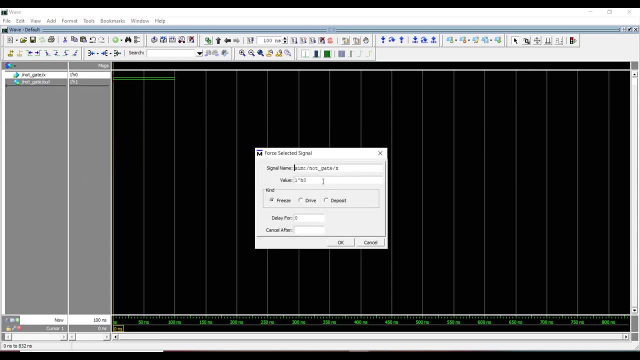 I'm getting is 1 and the run length, or the time period for what it has run, is 100 nanoseconds. you can see, for 499 seconds the waveform is there and then the value of the input. I'm going to do: change it to 1, run the code again. so now, 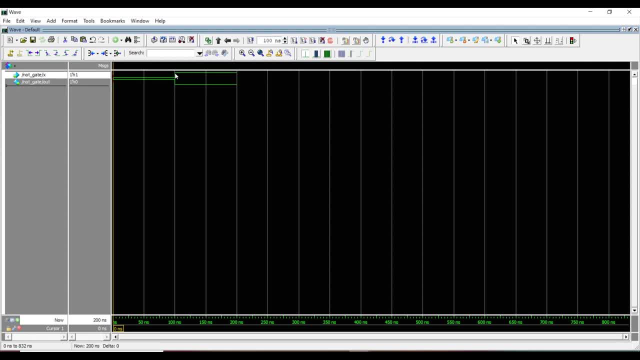 you can see the changes. also that when I have given input 1, it has gone up and the input is now 1 and the output has changed to 0. so now I can say that whatever code I have written here is correct. it is doing the function of a.